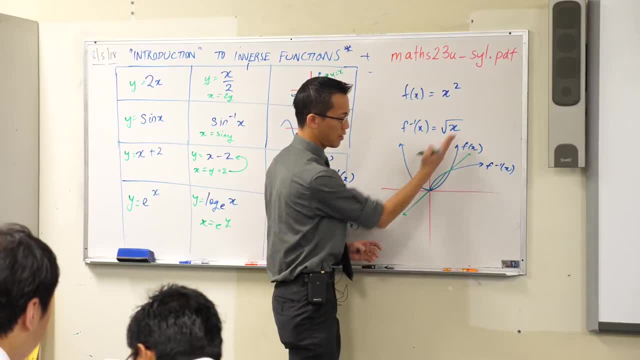 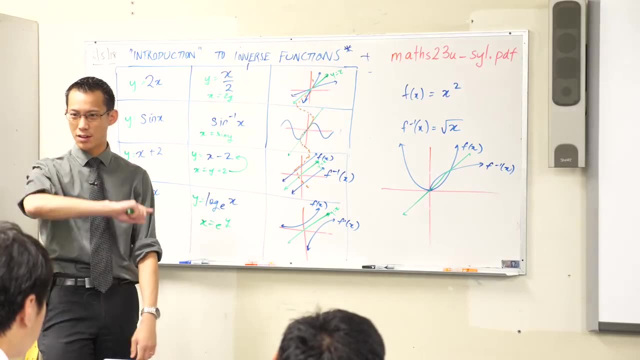 Across y equals x And you can see it sort of curves in, curves out. It's a really nice symmetry actually that I don't know if you've ever spotted before until it's highlighted for you. That's the first thing I want you to notice. 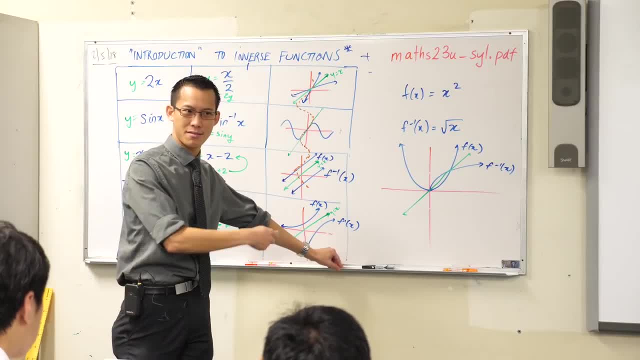 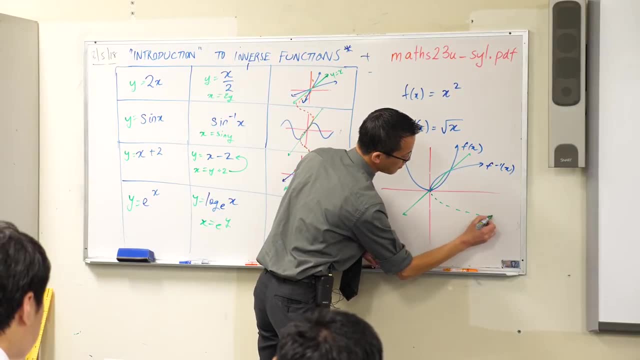 The second thing is: it's not a complete reflection, is it? It's a missing part. Which part is it missing? Where would it be if I reflected the whole thing? Yeah, it'd be down here. right, It would be down here. 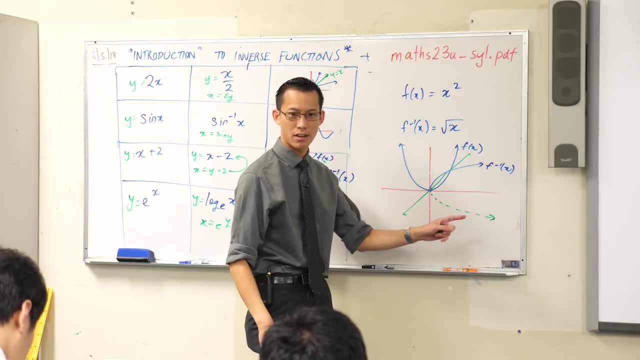 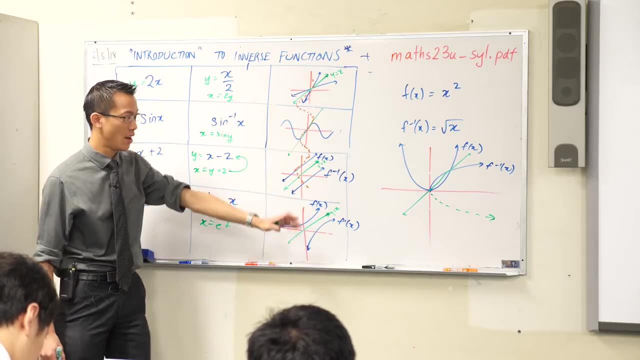 Why do we not have this guy down here? Why do we not have this guy down here? It's the same as the reason we don't have everything here in sine inverse of x. It wouldn't be this guy here if you included. it would not be a function, would it? 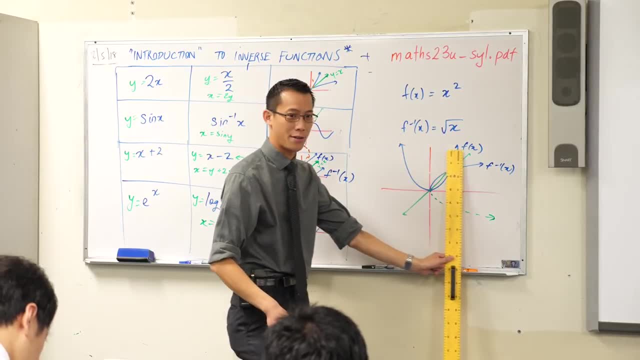 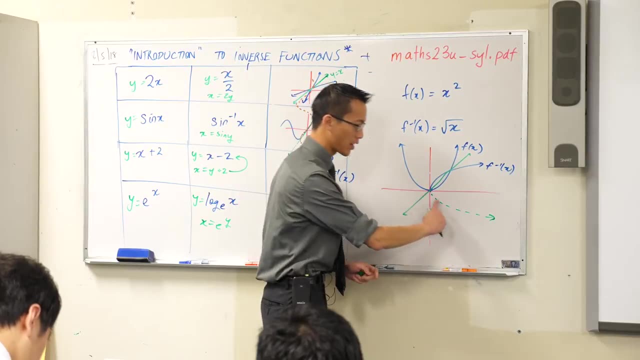 Because it would violate the vertical line test, like everywhere except for the origin. So because we want the square root to be a function, because that's useful to us, we say, oh, we're going to cut that guy out, We're only going to look at this particular part of f, of x. 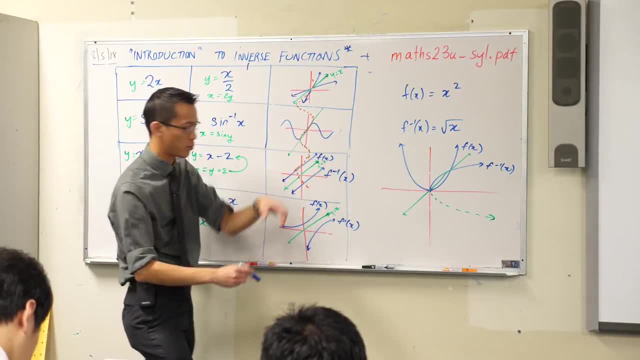 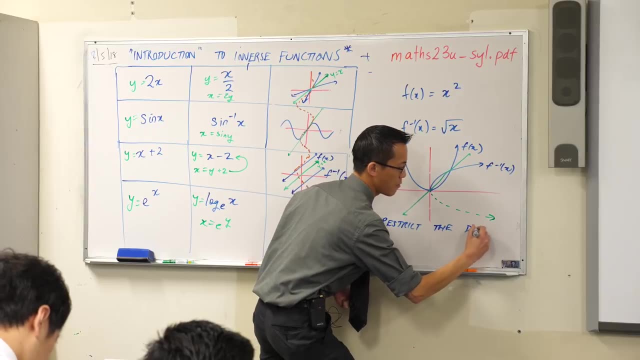 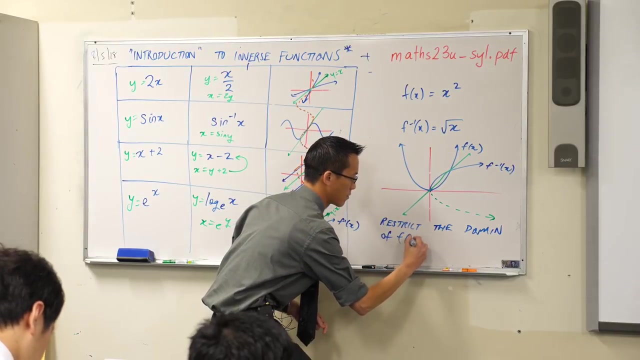 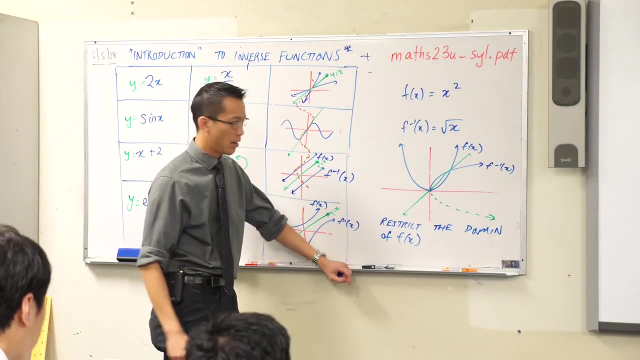 This is really important. We're going to write this down underneath where you've drawn, or beside where you've drawn this one. We restrict the domain. We restrict the domain of f of x, the original. What do we restrict it to? Which part of f of x do we look at and then reflect? 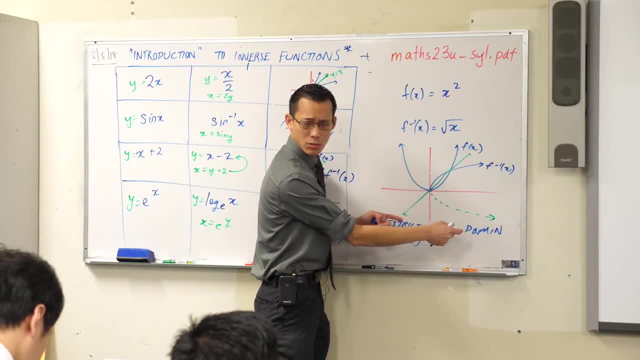 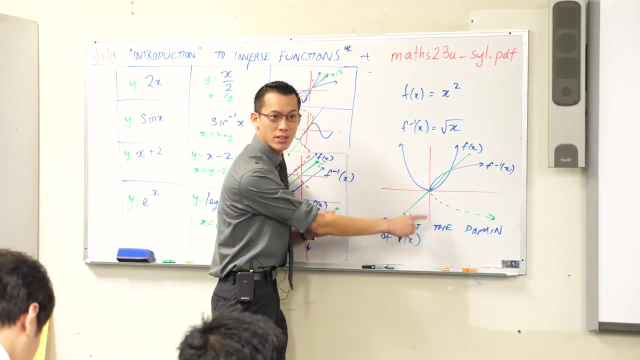 We look at I think it's domain right. Is domain x's or y's? It's x's, You can remember. it's alphabetical right Domain and range x's and y's. We restrict the domain of f, of x to x is. hmm, have a look. 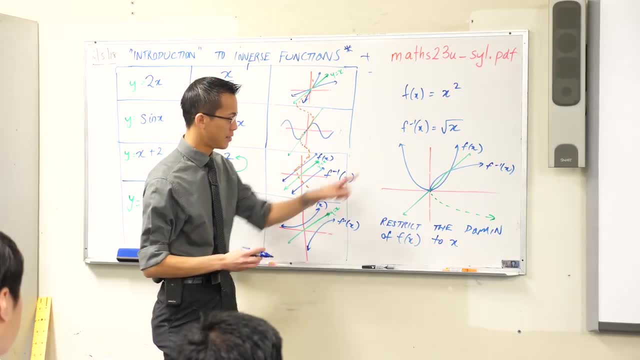 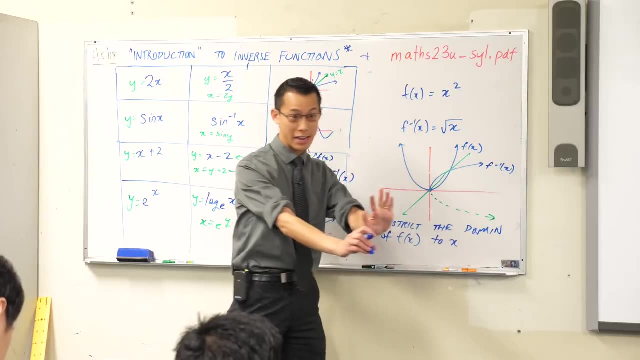 Which part gets reflected. Does this part over here get reflected? We want greater than or equal to 0.. We're okay with 0.. That guy's fine. So we're going to say x is greater than or equal to 0.. 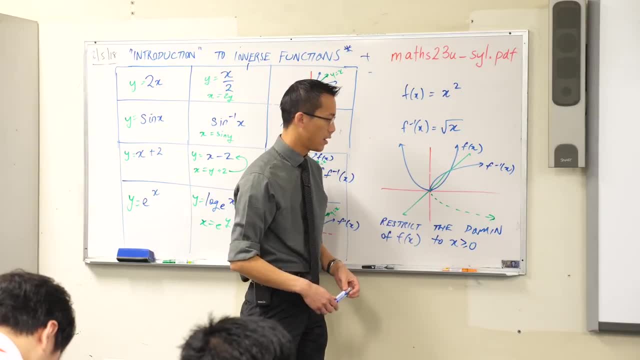 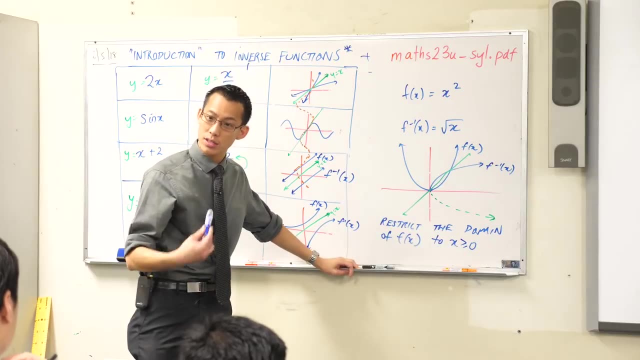 Okay, We chose that part and then we reflected it. Okay, Now, one of the weird things is, you didn't have to choose that part. We didn't have to. We could have looked at this part instead And we could still have reflected that. 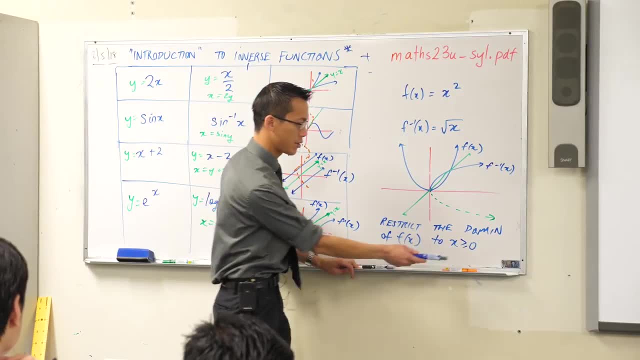 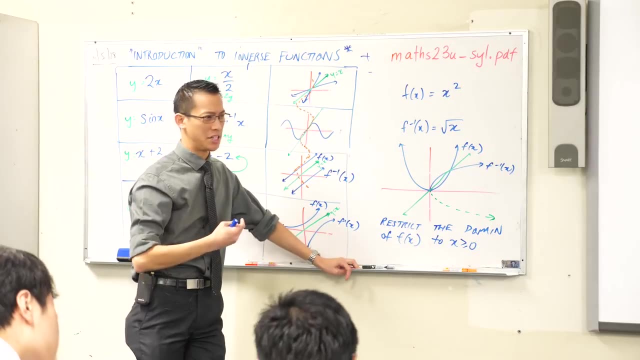 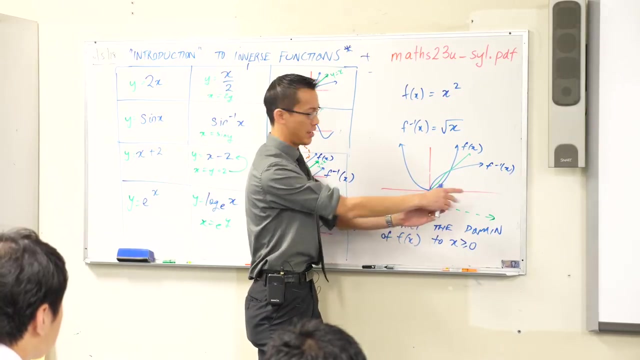 You would have still gotten a function. Why do you think we chose this part rather than the other side? It's positive, It's positive, I like positive numbers. But just because someone likes something is not a good reason to say: everyone everywhere and everyone's calculator should just be this part over here. 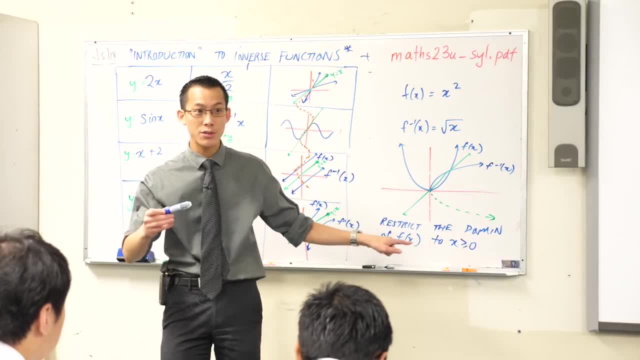 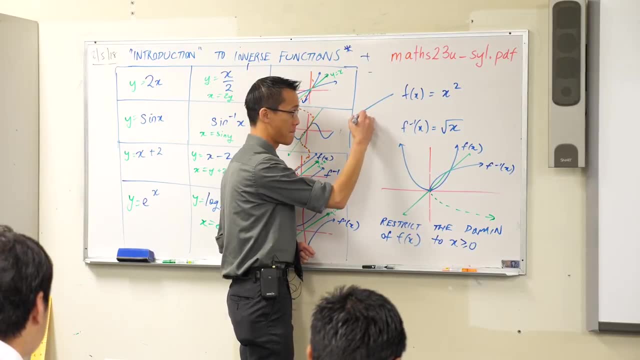 Or sorry, I should say this part over here. Why is this useful? I want to remind you again Where did we first meet square roots? We first met square roots when we were trying to work out: hey, you have a sign over here, right? 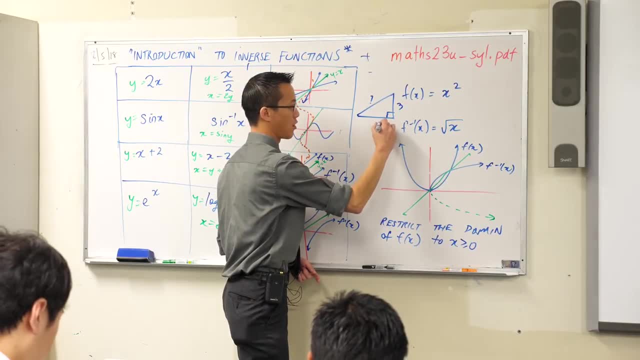 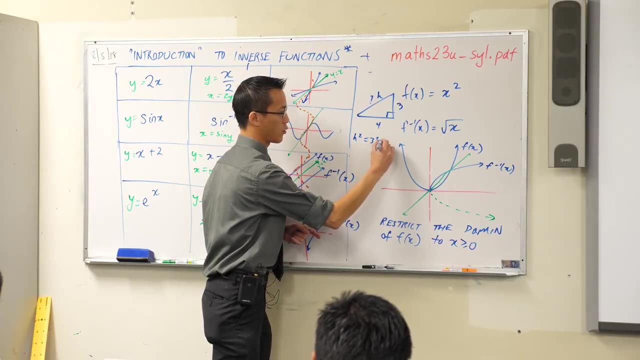 You try to find out what it is. You got 3.. You got 4.. And you would say, oh, that's going to be that hypotenuse there. right, That'll be: h squared equals 3 squared plus 4 squared. 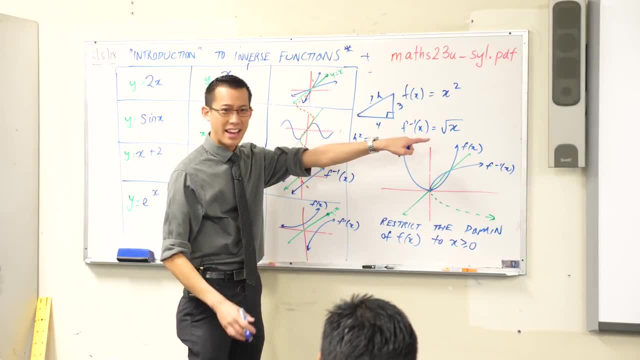 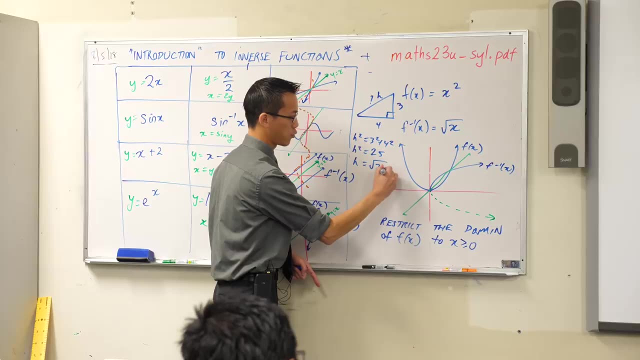 And you have to invoke The square root function right Now. it would be kind of weird if we said: well, h squared equals 25.. h is going to be the square root of 25.. Oh, that's restricted to the negative value. 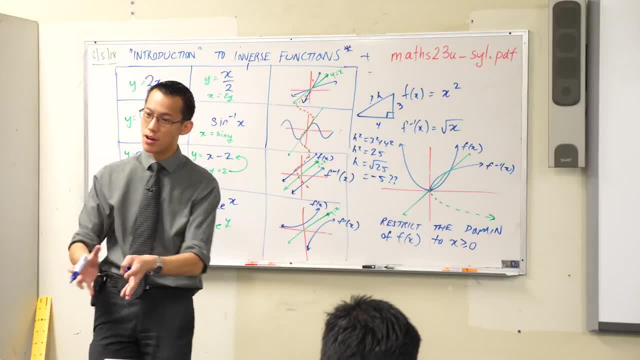 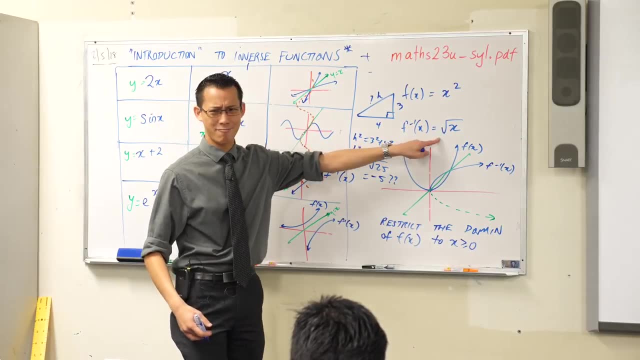 That would be really weird, right? Square roots emerged in the context of measurement, And in measurement, things are positive, Yeah. So therefore, if I'm going to get, if I want, positive values out of this, I might as well restrict it to the positive values. 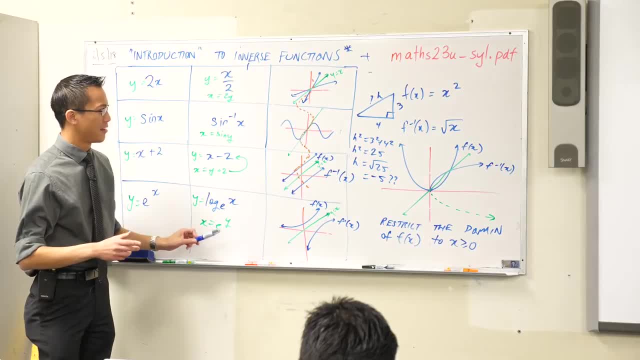 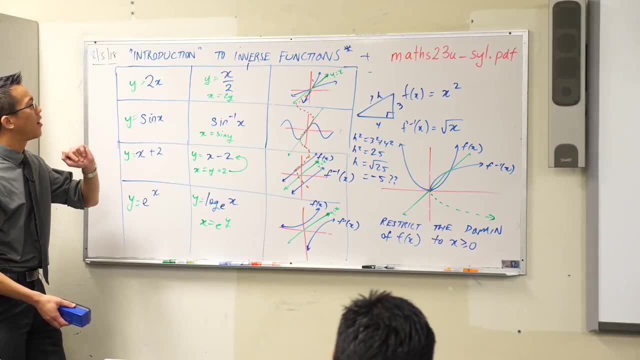 Does that make sense? OK, I need more space to point out one more thing, and then we're going to let you have a go at actually using these things and manipulating them. OK, I said right at the beginning: let's run off this side here. 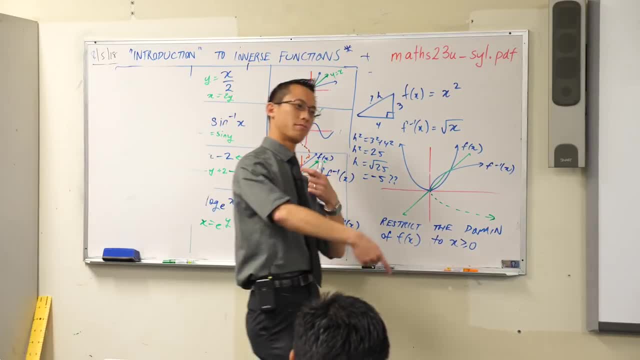 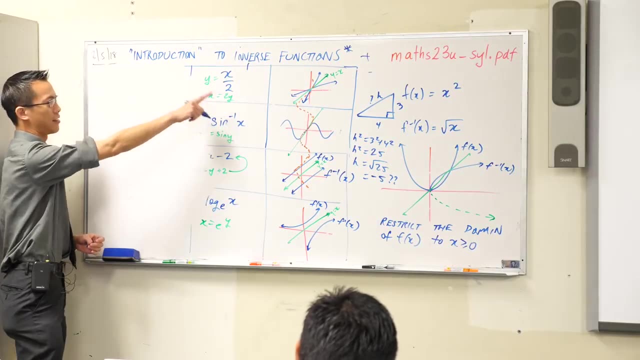 I said right at the beginning that an inverse will just sort of reverse the direction or turn something inside out upside down. OK, So therefore you can do one last fancy algebraic trick with something like an inverse right If you have a function like addition right. 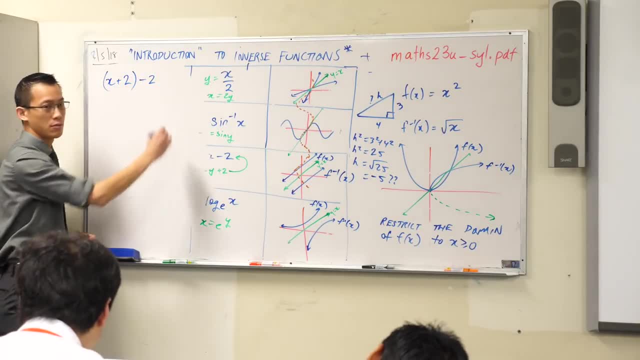 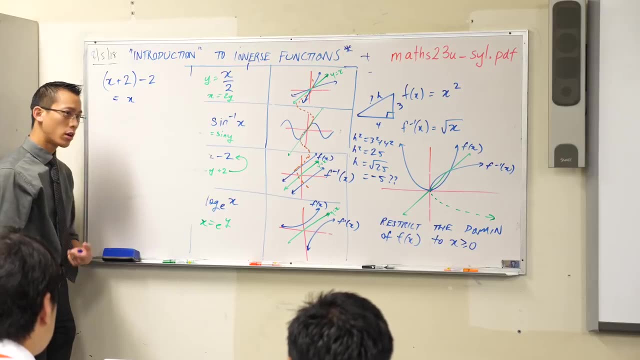 And then you apply that, And then you apply the inverse, which is subtraction. What do you get out? the other end? You just get. well, these two things, they cancel. so you get x Right. What if you did it with multiplication?